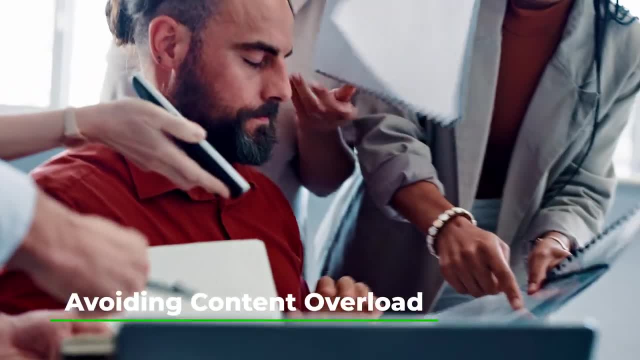 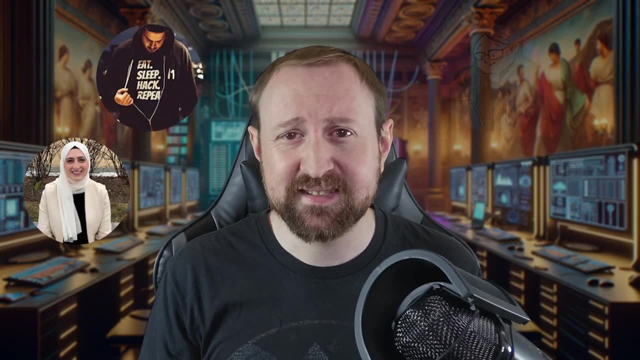 let's jump right in. It's very easy to get overwhelmed by the amount of application security content out there. There are so many great content creators like Rana Khalil Nahamsek, InsiderPhD and LiveOverflow, to name just a few. You don't need to watch. 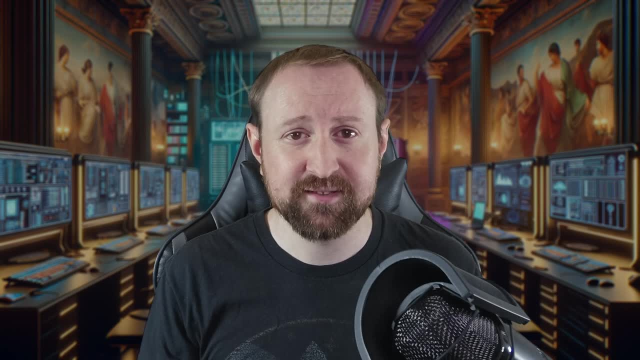 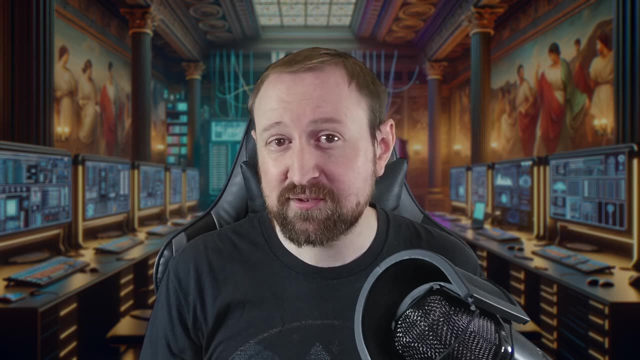 every video someone puts out, especially if you feel it might be too advanced or if it covers some area you already know about or aren't interested in. The same goes for blog posts, podcasts and live streams. What I do recommend is creating some form of rich text document. 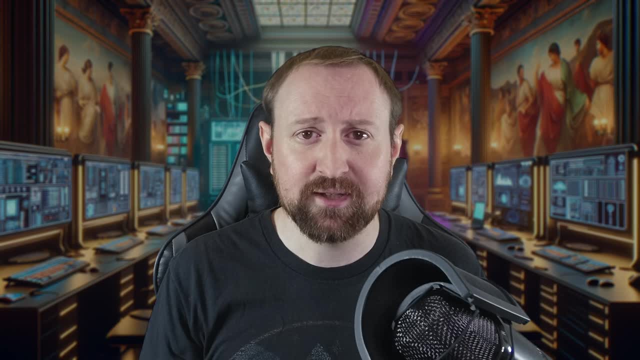 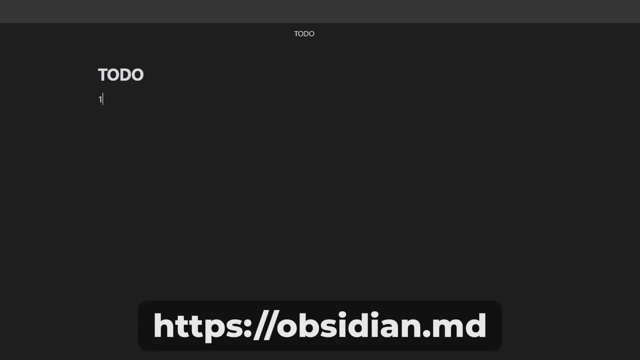 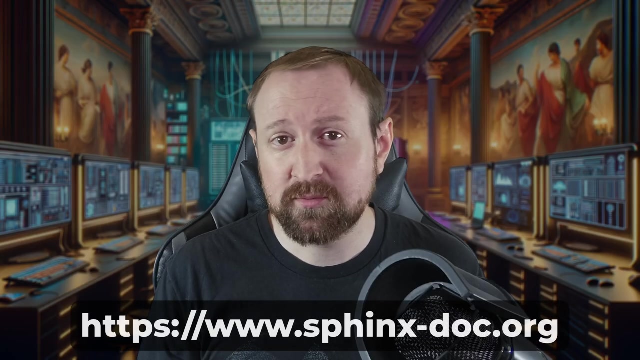 where you can paste links to content you think might be useful later on, or even payloads and techniques for specific vulnerabilities, even the rare edge cases. I've seen people use Obsidian because it uses Markdown, which is super simple to pick up and the document is made up of simple text files. I personally use Sphinx. 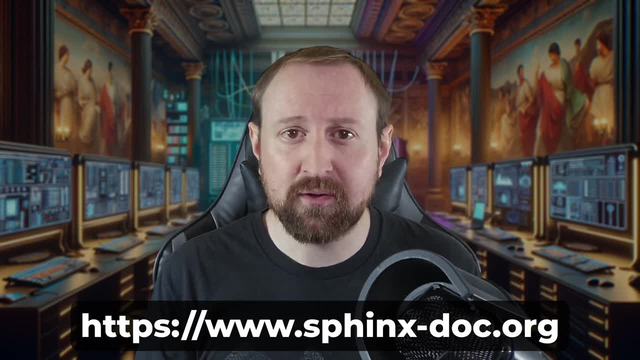 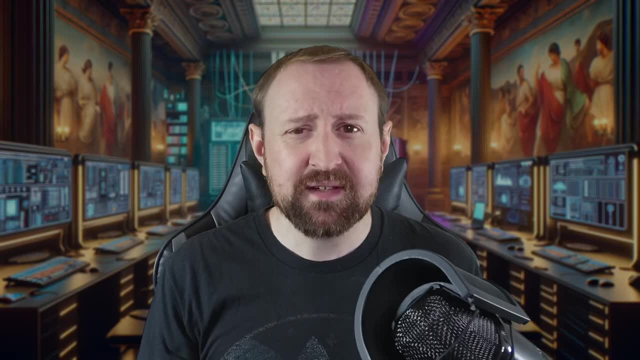 which uses a similar language to Markdown. However, I can compile the document into a PDF or even into HTML so it can be opened in a web browser. While some people might have amazing memories, for most of us, mere mortals, it's just not possible to remember everything. 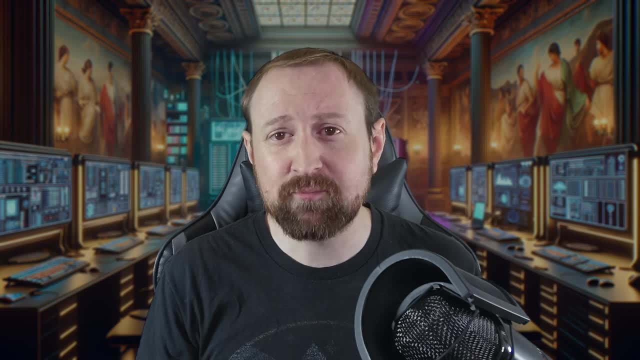 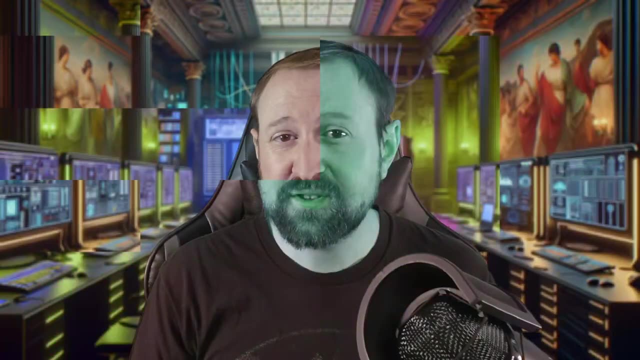 especially in AppSec. Writing your own notes not only helps retain a general understanding of certain concepts, but it also means you have reference materials that you can use to create materials on hand, so you don't need to search the internet If you're serious about a career in. 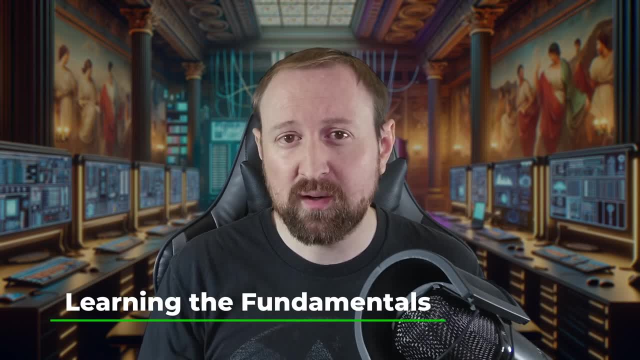 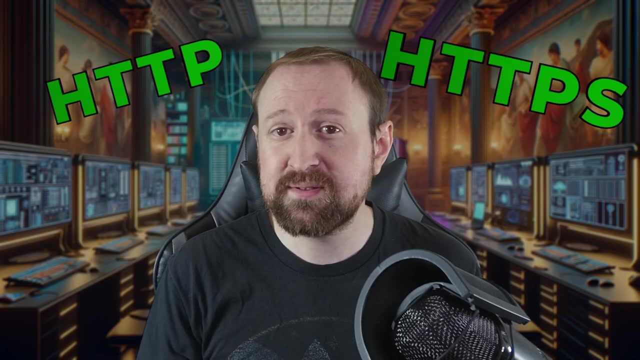 AppSec. you need to learn the fundamentals- how web applications work and the underlying technologies that hold them together. This includes protocols like HTTP, HTTPS and even WebSockets. if you want to get advanced, You should also know about client-side technologies. 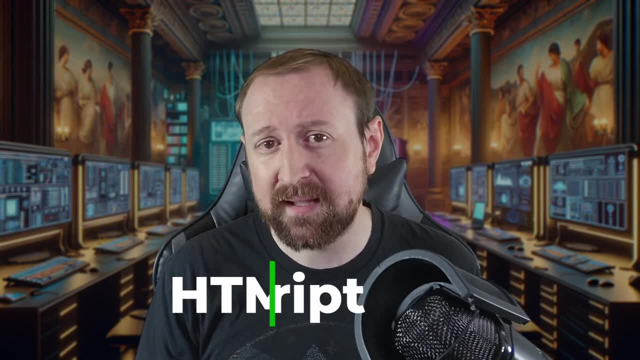 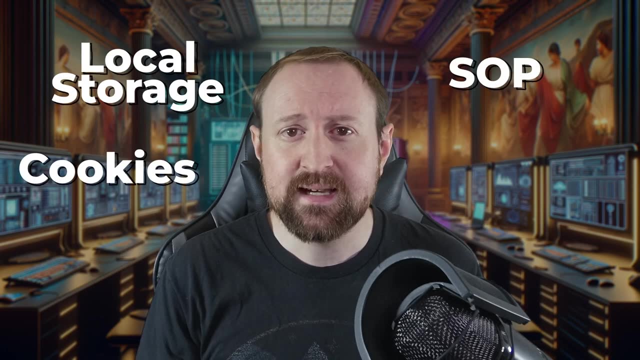 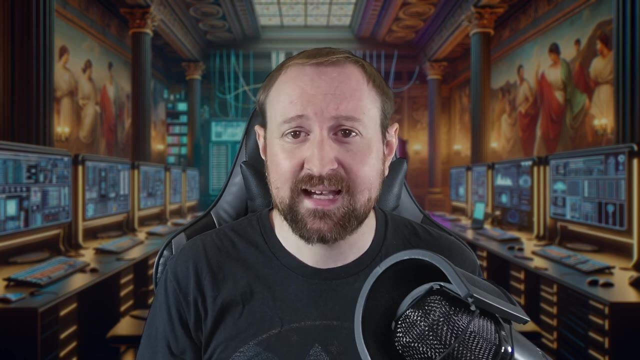 how browsers work and the basics of languages like HTML and JavaScript. It's also a good idea to learn about cookies, local storage and concepts like the same origin policy and cross-origin resource sharing or CORS. Finally, it's important to learn about server-side technologies, such as web servers and databases. The Traversy Media channel on YouTube. 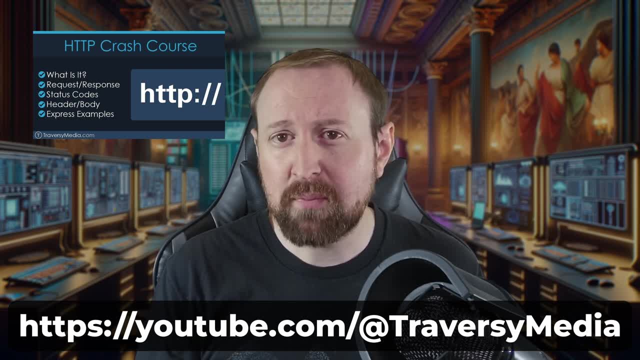 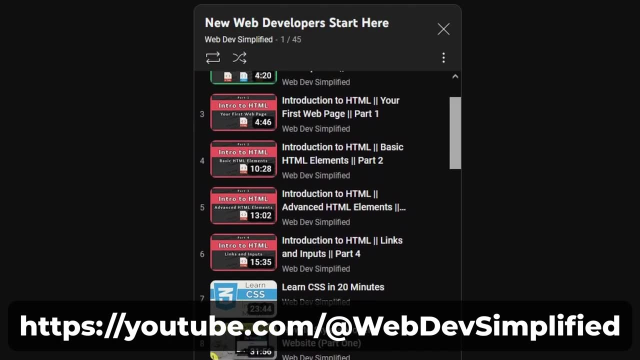 has a great crash course not only on HTTP, but also both client and server-side technologies. Similarly, WebDev Simplified has several short 5-10 minute videos covering the basics. Maybe watching videos isn't how you learn. That's fine too. I've learned a lot about web application. 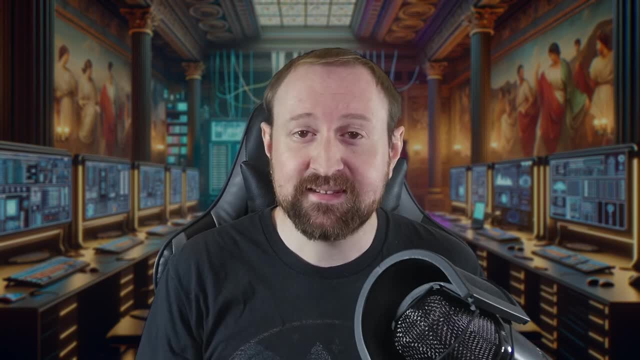 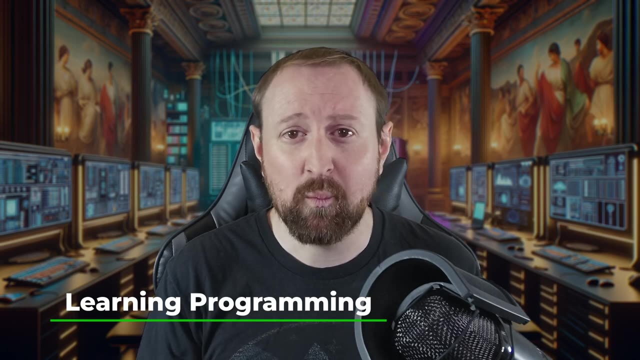 technologies from Wikipedia, for example, And if you're interested in learning more about web applications, you're feeling particularly daring. you could even crack open an RFC. I get asked all the time if it's important to learn programming if you want to be a web app. 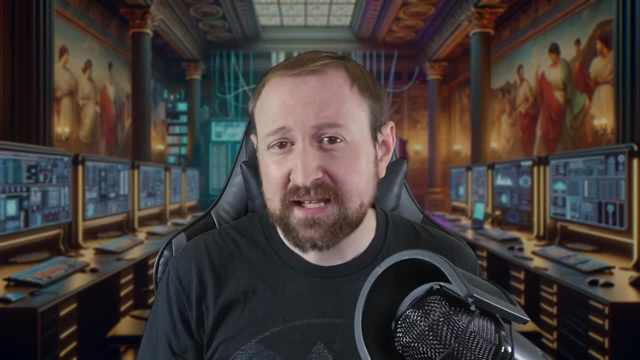 pen tester or bug bounty hunter. My answer has always been that you can definitely do the job without being proficient in a programming language, but you're ultimately shooting yourself in the foot. Please note: there's a big difference between being able to read code and being able to write it. 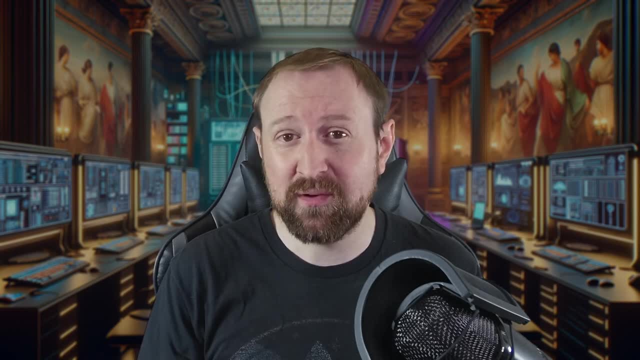 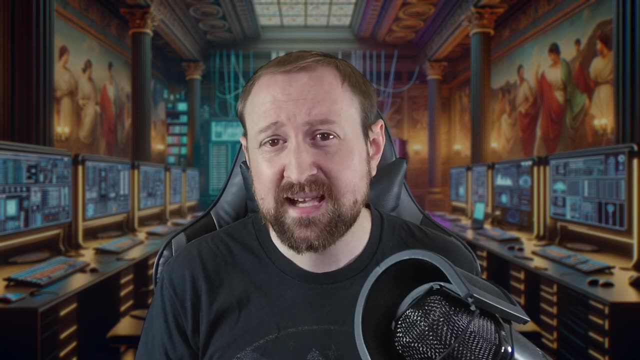 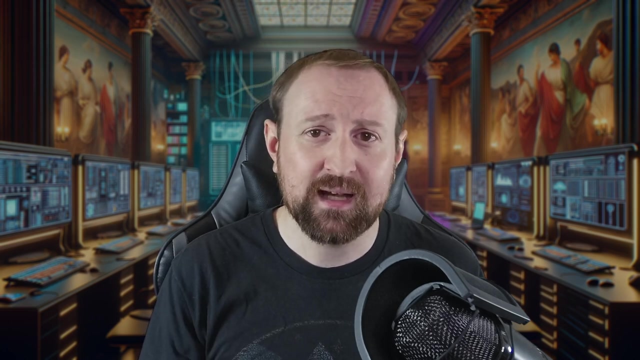 If you've covered the fundamentals already, you should at least be familiar with HTML and JavaScript code. Reading code allows us, as testers, to learn the basics of web applications. It will also help you craft client-side payloads like cross-site scripting, since often you'll have 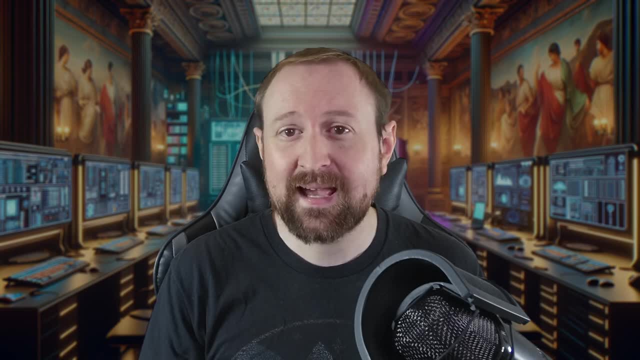 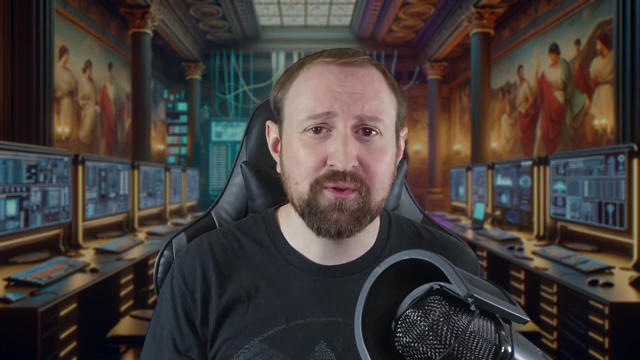 to understand the code context you're injecting into. However, I cannot stress enough how being able to code in at least one programming language can benefit your AppSec career Personally. there's the automation aspect: Being able to write code to perform repetitive tasks. 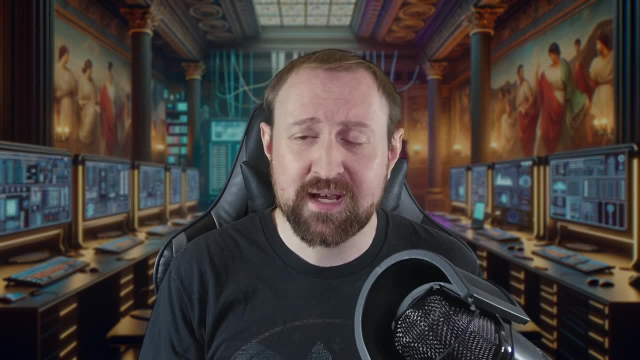 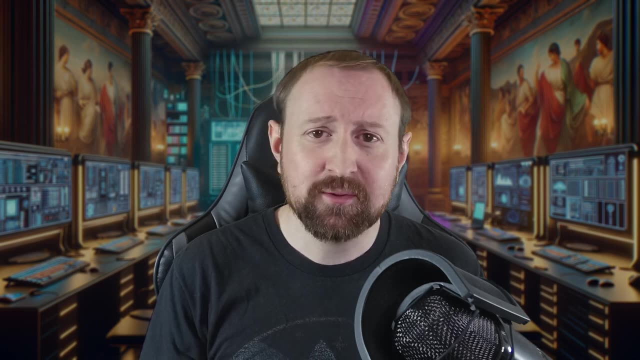 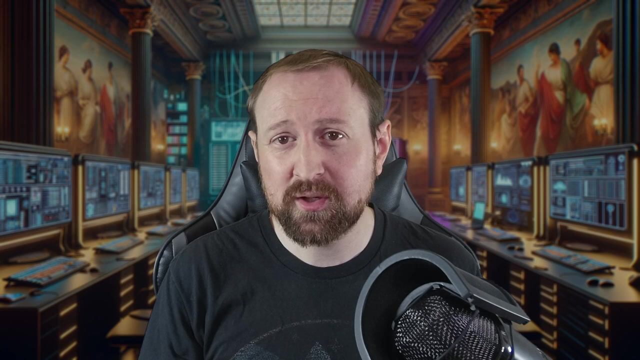 saves so much time, especially since you can often repurpose your code in future engagements. At a deeper level, you can use your programming knowledge to create web applications of your own and use these to enhance and test your understanding of fundamental web application concepts. You can also purposefully use insecure code. try out new testing techniques. 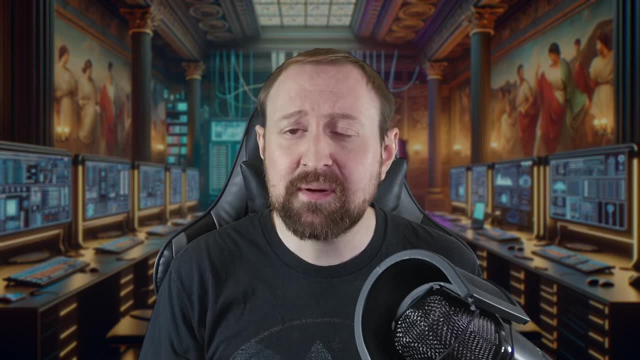 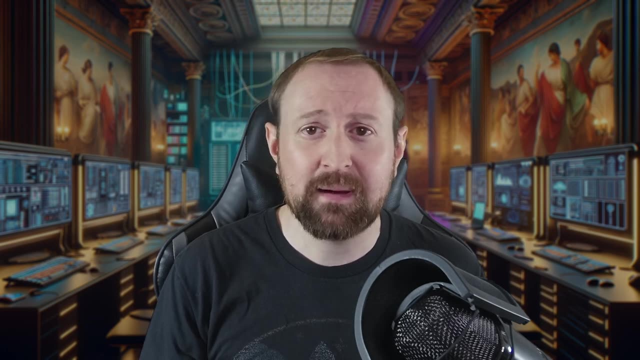 and see how different mitigation strategies affect the result. Remember, you're not trying to become a full-stack developer, but during your AppSec career you will be talking to developers, so being able to talk about things from a developer's perspective is so important. As for what programming language you're going to use, you'll need to be familiar with the programming language you're using. You'll need to be familiar with the programming language you're using. As for what programming language you're using, you'll need to be familiar with the programming language you're using. 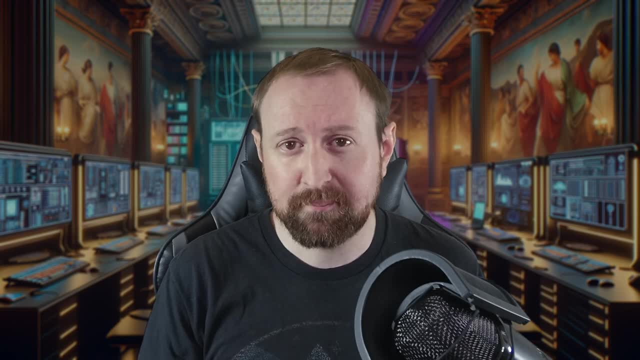 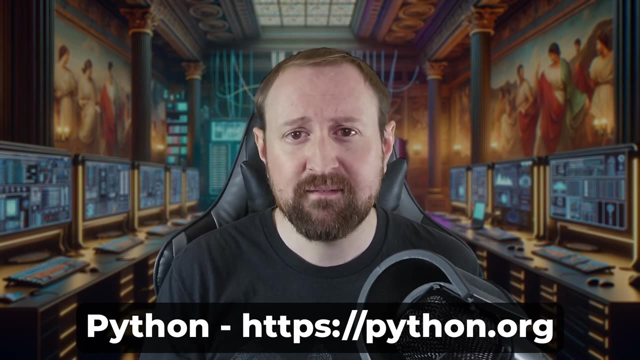 I would recommend, at the very least, you become somewhat proficient in Python. Python is a versatile language that does not require a compiler, meaning you can code and execute simple scripts very quickly. It's also usually installed by default on many Linux distributions, as well as MacOS. 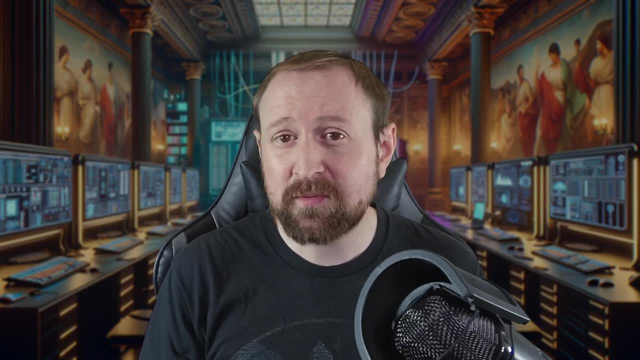 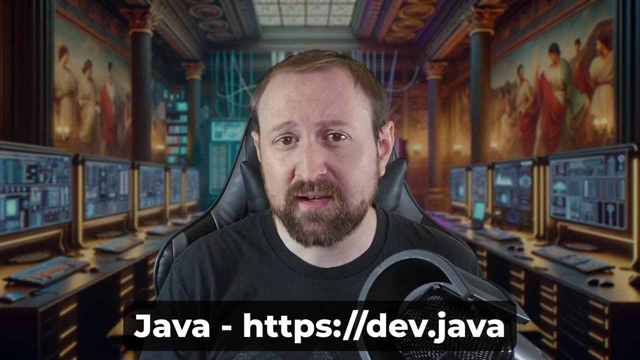 If you're serious about becoming a web application pen tester, I would also recommend learning Java. The reason for this is that the main testing tool most web app pen testers use, Burp Suite, is coded in Java, and modern Burp Suite extensions need to be written in Java as well. 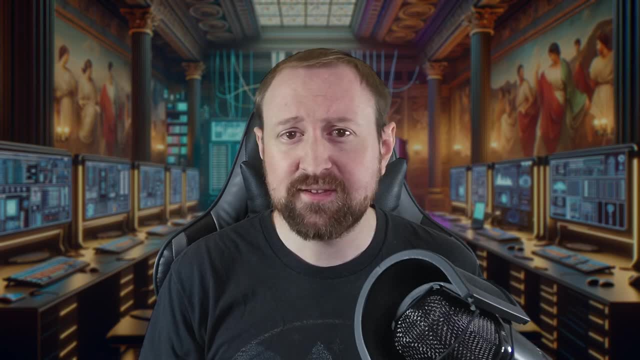 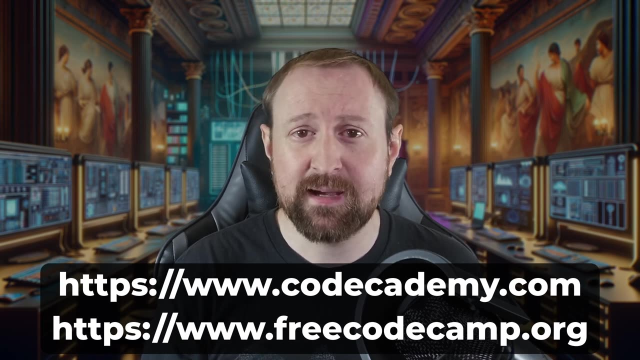 There are many places where you can learn how to code for free. however, the two most popular places are Codecademy and FreeCodeCamp, so check those out If you're a TCM Academy subscriber or are planning on getting a subscription. we also have Python for Hackers courses. 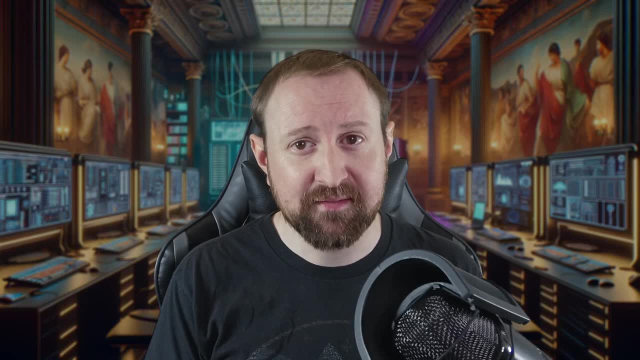 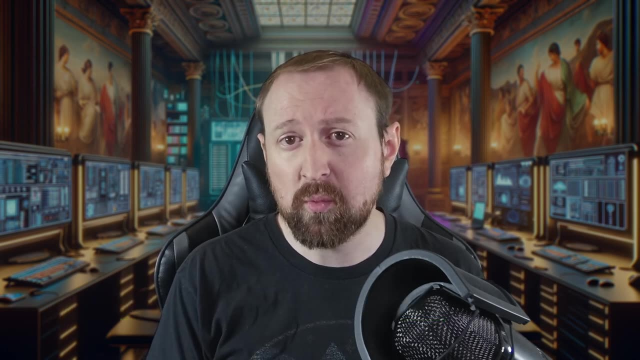 So far, we've covered the app of AppSec, so we should probably talk about the Sec. You'll need to learn lots of security concepts specific to web applications, such as the different vulnerabilities, including why they occur, how they can be detected, exploited and ultimately mitigated. 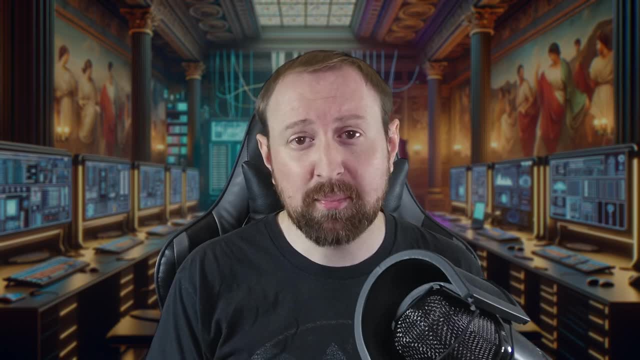 Another important thing to learn is various testing techniques, how to properly enumerate an application, which parameters look interesting and have a greater chance of being vulnerable and, ultimately, how to use fuzzing and scanning techniques combined with manual input and analysis, to determine if a vulnerability exists. 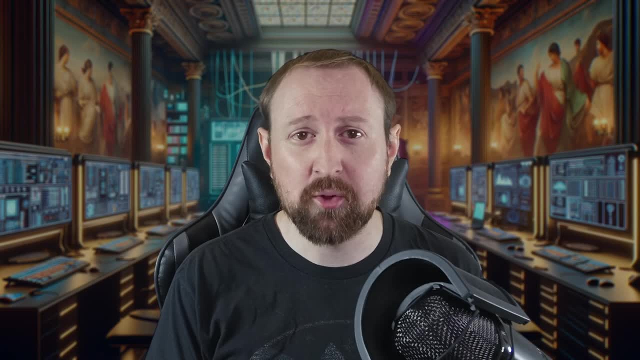 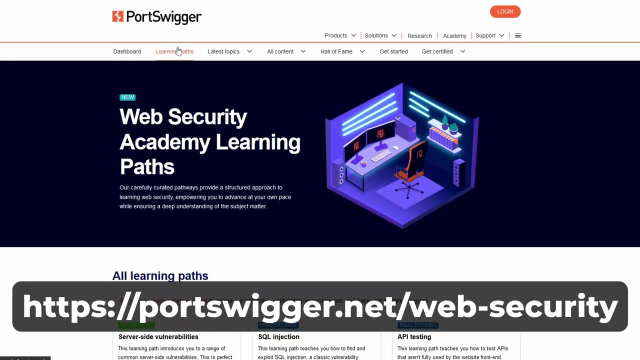 There are so many great resources out there it's hard to narrow it down to only a few. However, I highly recommend signing up for a free account over at Port Swigga web academy, where there are several learning paths and individual topics that cover the most common. 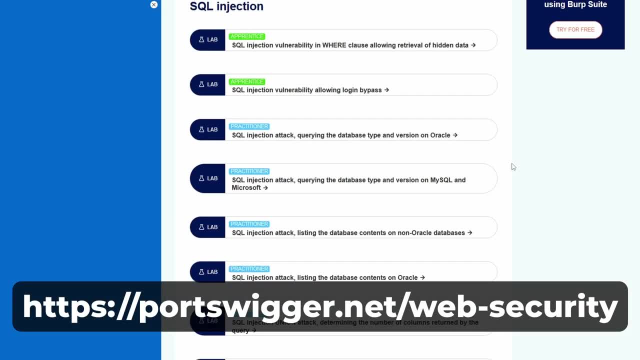 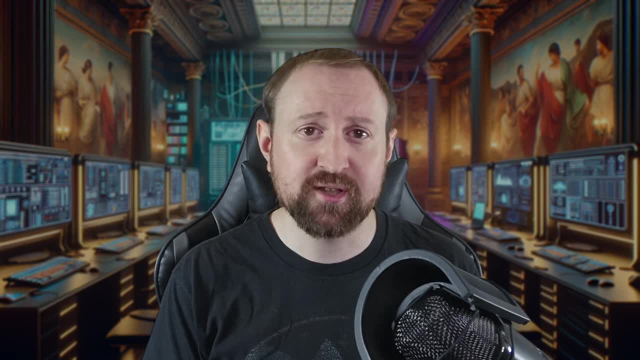 vulnerabilities. In addition to this, there are over 200 labs with different difficulty levels for you to practice Again. this is a 100% free resource. OWASP, the open worldwide application security project, has a free cheat sheet series and web security testing guide which covers the 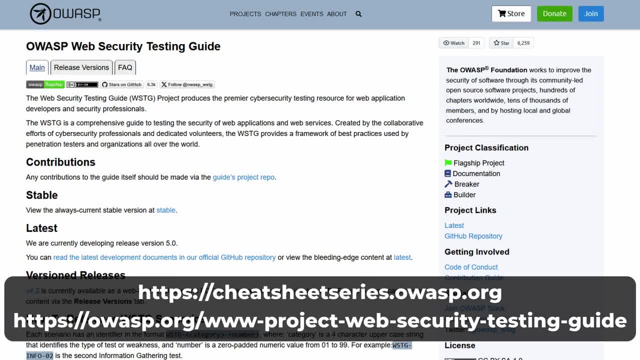 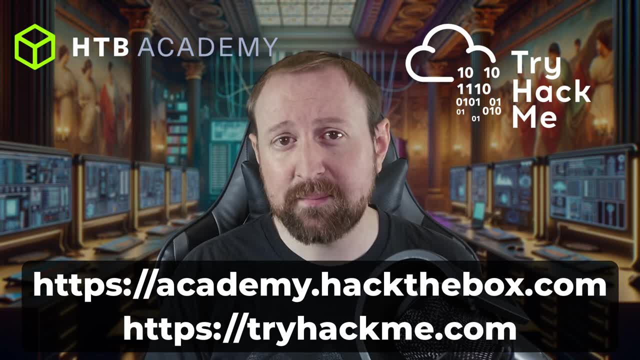 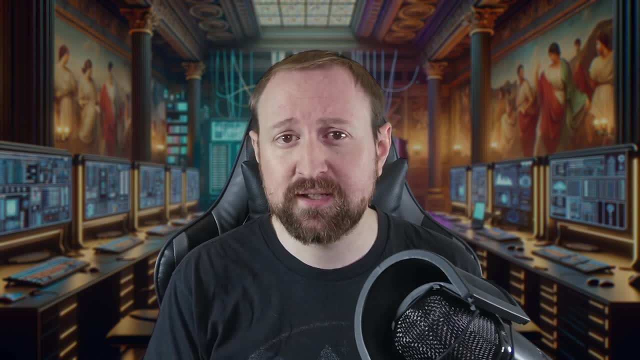 full testing process and provides useful tips and techniques for finding vulnerabilities. If you're prepared to spend a little money, then both Hack the Box Academy and TryHackMe have additional courses and learning paths with live practice web apps to try your skills against. Of course, at TCM Academy we also have several application security courses. 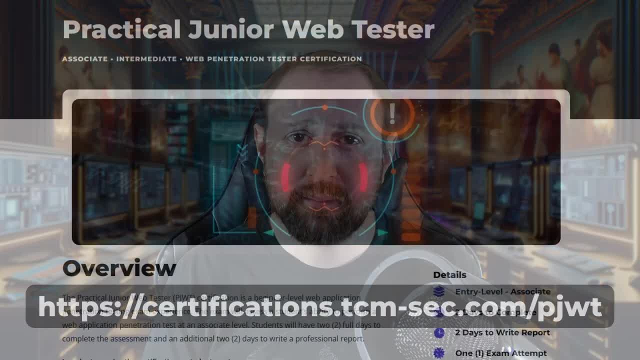 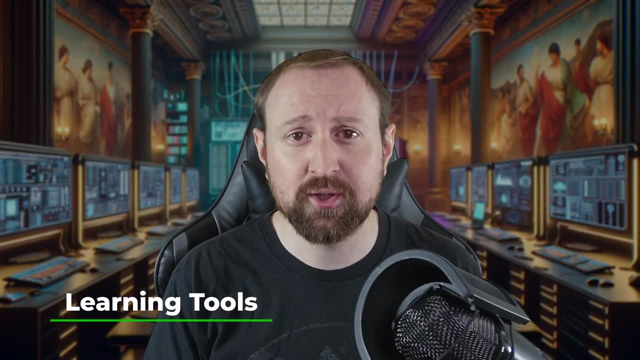 such as Practical API Hacking and Practical Bug Bounty, plus the new Practical Junior Web Tester certification. There are hundreds, if not thousands, of tools available for testing the security of applications. however, one shines brighter than the rest: Burp Suite Pro, The paid version of Burp. 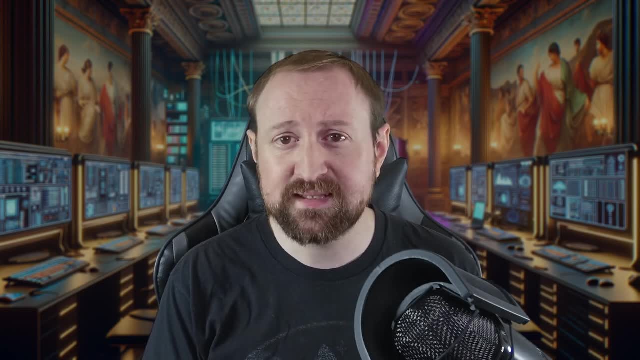 Suite contains almost everything you need to find and exploit vulnerabilities in web apps and apps that you can't find anywhere else in the world. You can use it to find and exploit bugs and is the main tool of web application penetration testers. The documentation for Burp. 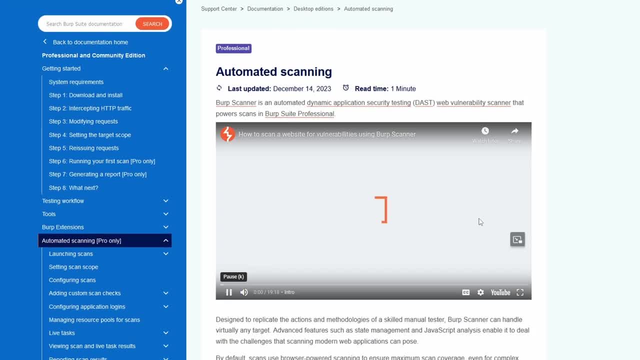 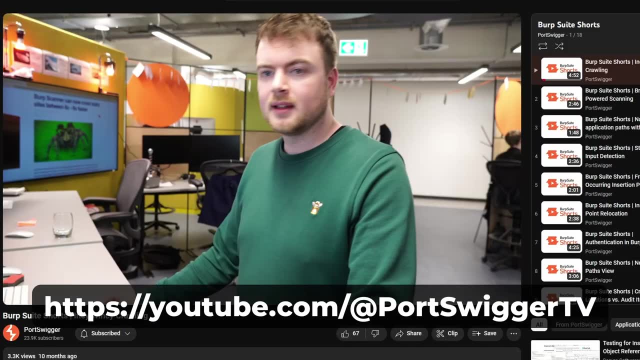 Suite is well written and has video walkthroughs explaining various features and testing techniques. In fact, the Portswigger YouTube channel is worth subscribing to, as they have started releasing short videos when new features are released. TryHackMe has a Burp Suite module available. 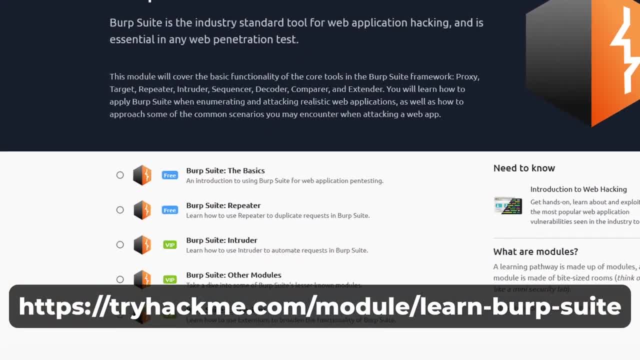 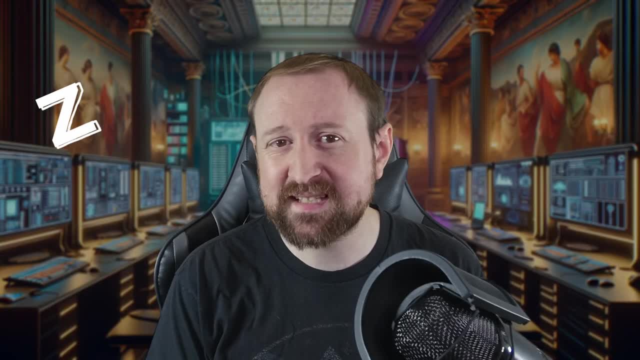 which teaches you how to use Burp against live examples, with two rooms available for free users and three extra rooms only for subscribers. I know people watching will be thinking: what about Zap or Kaido? and if you've watched my streams before, you know I'm personally not a fan of either. however, I do recognise both are quickly adding features and in 2024 they may start catching up to Burp Suite. in terms of functionality, Zap is 100% free, which makes it a great option to try if you're just starting out, whereas Kaido costs $100 a year. Burp Suite. Pro, on the other hand, is currently $449,, though if you work as a pen tester, you will almost always get the license provided to you by your employer. Burp Suite Pro, on the other hand, is currently $449,, though if you work as a pen tester, you will almost always get the license provided to you by your 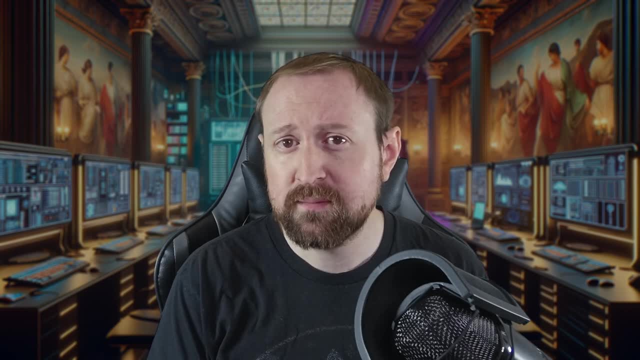 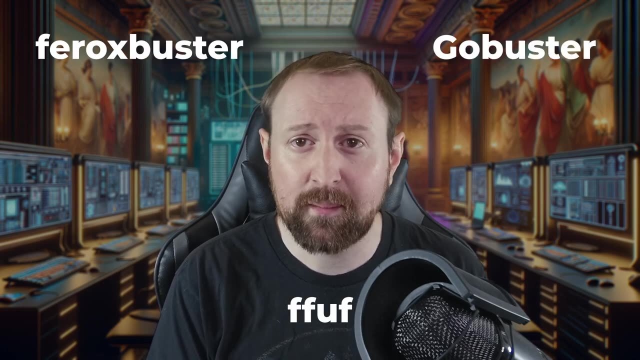 employer Other than Burp Suite. you may wish to learn a directory busting tool. Again, there are a fair few available, like Ferox, Buster, Go Buster and even FFUF. This will help with the enumeration stage of web application hacking, identifying hidden files and. 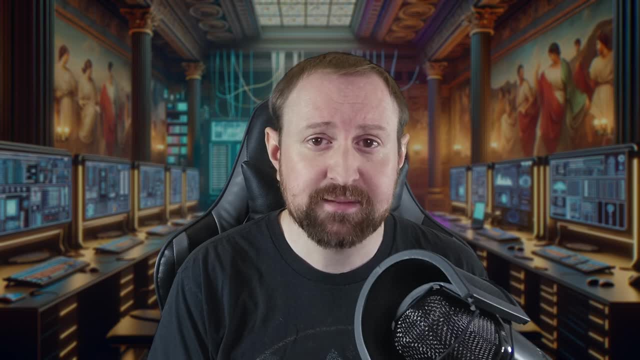 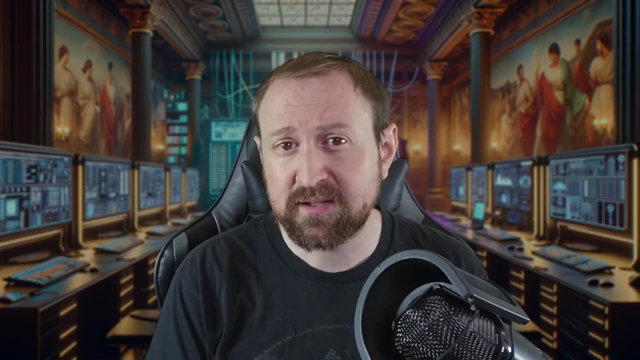 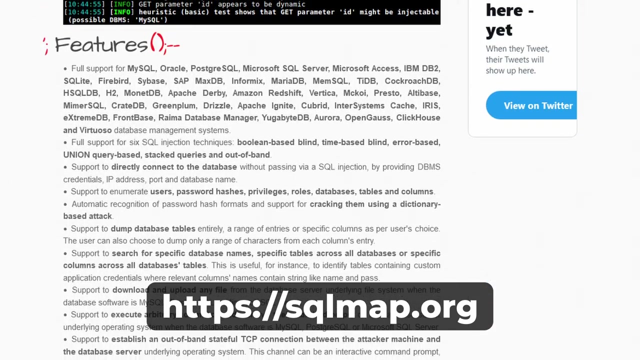 functionality which are easy to miss. Several vulnerabilities have inspired highly specialised tools aimed at making their discovery, and often their exploitation, far easier to achieve. For example, SQL Map is pretty much the best tool for finding and extracting information from web applications, making this often slow, manual process almost entirely automated. 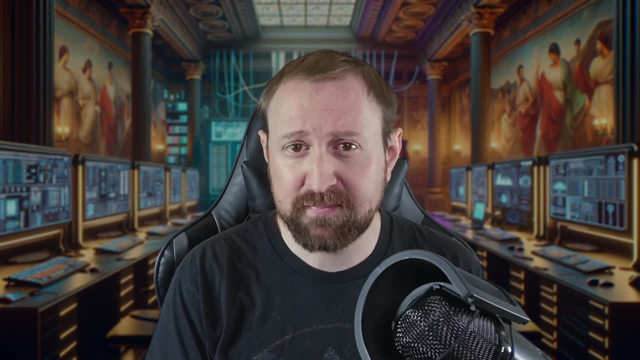 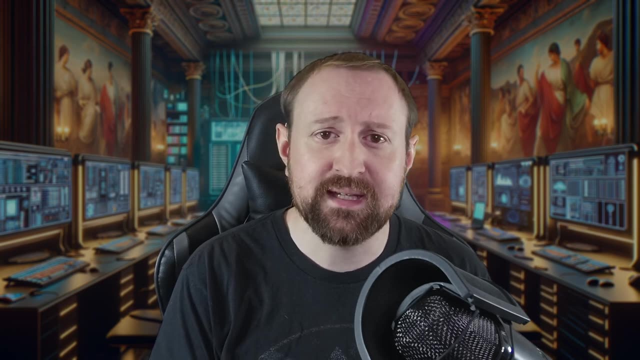 It goes without saying that you don't need to be an expert in any of the tools I've mentioned to start your career in AppSec. In fact, you can often learn the basics and then gradually expand your knowledge when you encounter the need for certain features or tools themselves. 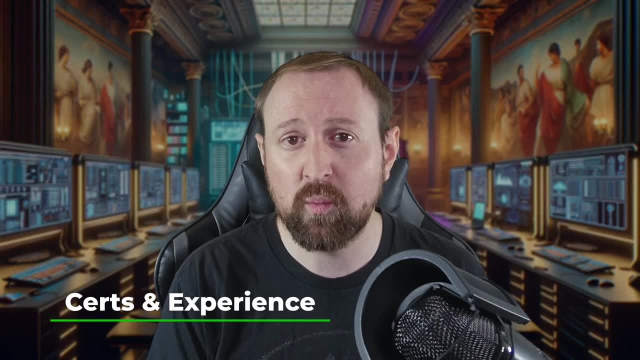 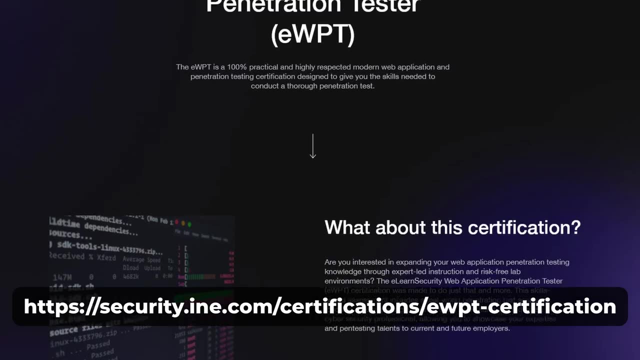 There are a few AppSec certs out there, including the Practical Junior Web Tester from TCM Academy I mentioned earlier. but eLearn Security also have the eWPT and, more advanced, eWPT-X. Hack. the Box Academy have their certified Bug Bounty Hunter cert, which is aimed at entry level. 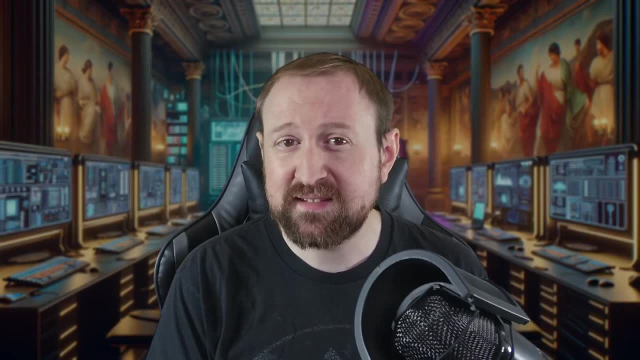 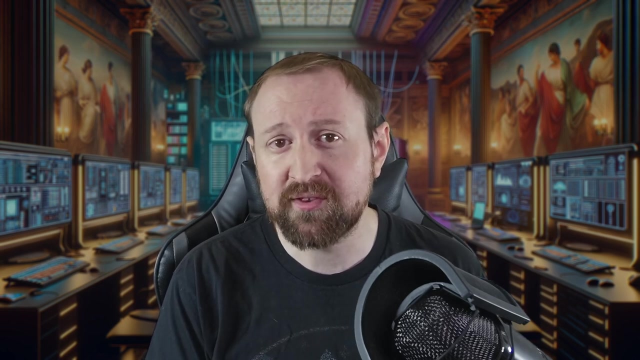 bug bounty hunters and web app pen testers. Speaking of bug bounty, this is a great way to gain real world experience and improve your skills. There are several bug bounty platforms available, with the main three being HackerOne, Bug Crowd and Integrity. Most platforms are open to newcomers and if you follow the stated rules of both the platform. 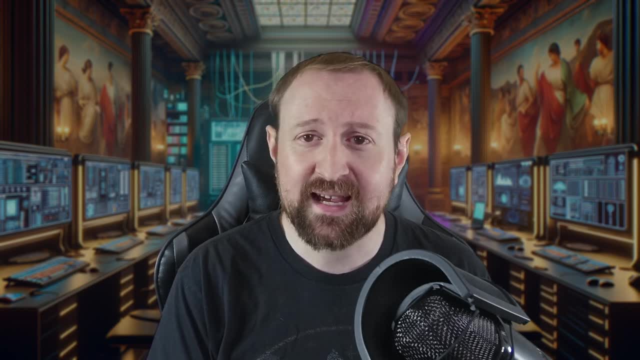 and, more importantly, the bug bounty program. you can try your hand at hacking live sites without legal repercussion. If you're interested in learning more about bug bounty, check out the link in the description below. In addition, these platforms are great places to hone your skills at writing. 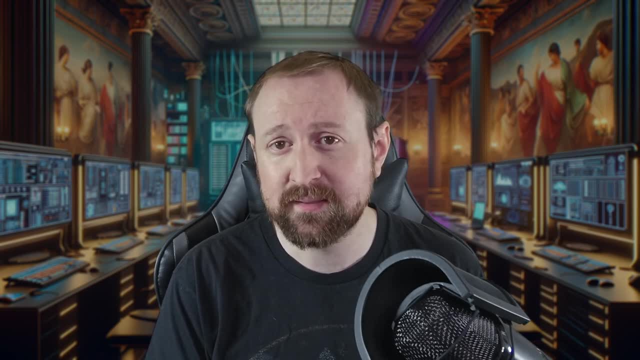 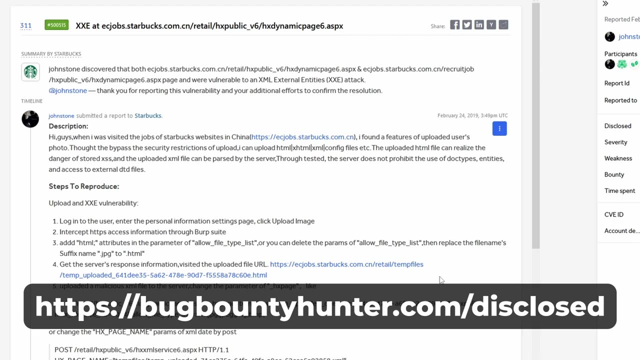 reports, which is key if you want to transition to pen testing at some point. I highly recommend reading publicly available bug bounty submissions to see the level of detail which goes into these reports and try to match that level of detail yourself. A really useful site I've been using. 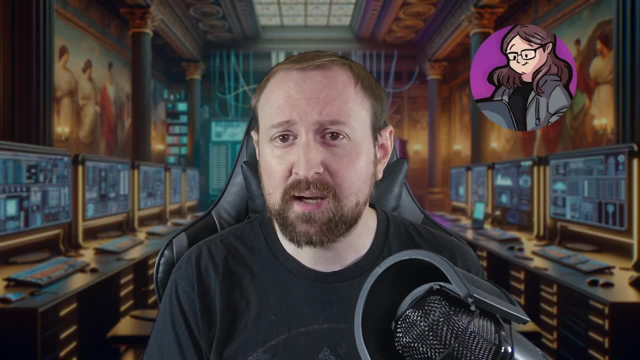 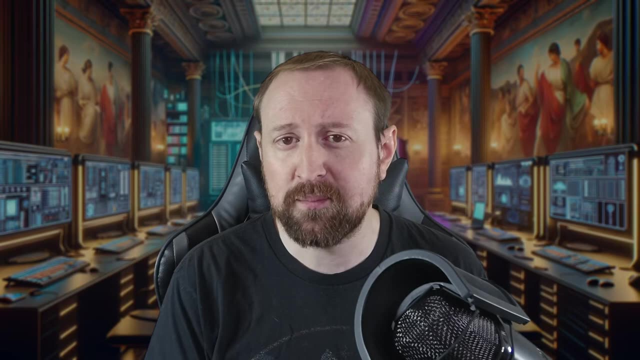 recently on the recommendation of Insider PhD, is Bug Bounty Radar. It updates every five minutes with the latest bug bounty programs added to 10 different platforms. Since you only get credit if you find the bug before anyone else, being among the first to start testing on a program gives you. 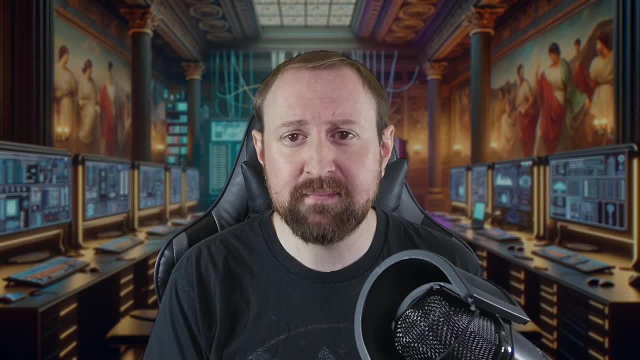 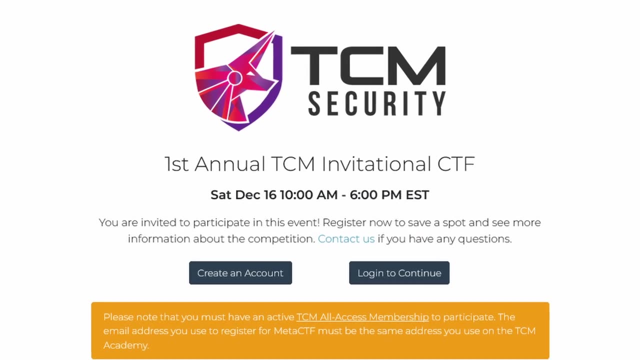 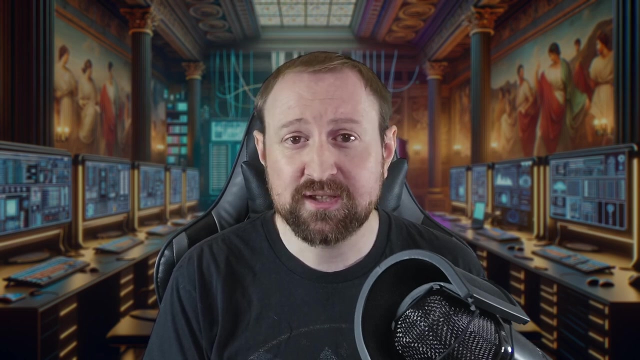 a significant advantage. A final avenue of experience worth mentioning is CTFs, or capture the flags. These are events often hosted by security organizations, including many conferences, where the goal is to solve security related puzzles. Although each CTF is a competition between many teams, you can enter just for the fun, either solo or with some friends. 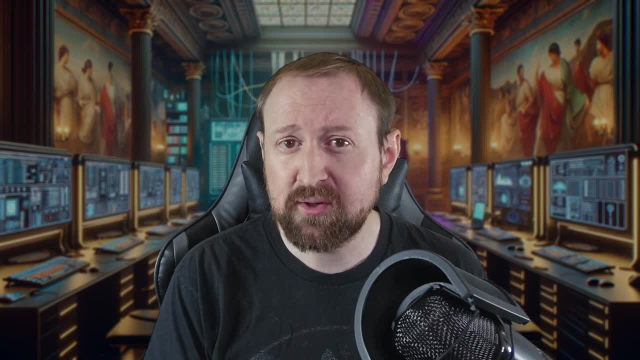 Web-based challenges are common and often range in difficulty. In most cases, the challenges aren't 100% realistic. however, they will still feature standard vulnerabilities, usually with some twist. you need to figure out. The best site to find upcoming CTFs is CTF Time. 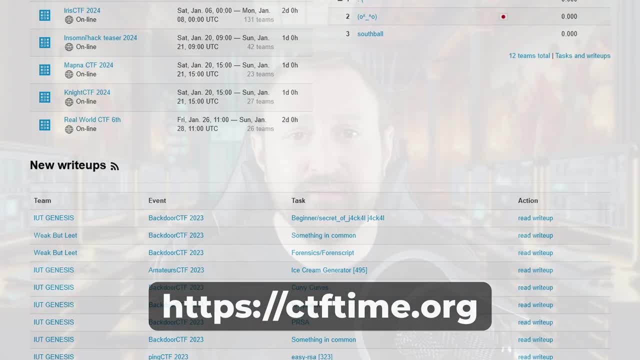 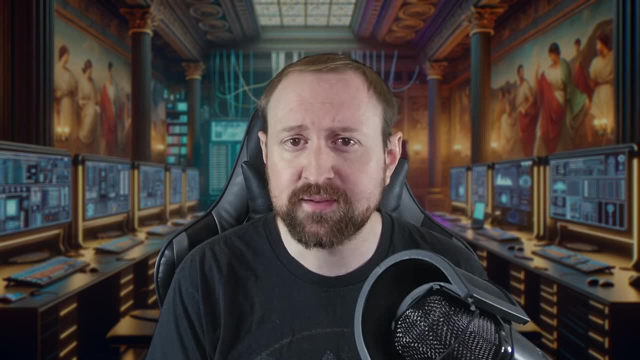 If the CTF has an associated forum or Discord server, you may even find teams looking for an extra player. Even if you don't figure out a challenge, the top teams usually post walkthroughs on CTF Time afterwards. These are worth reading to learn tips and tricks for approaching challenges. 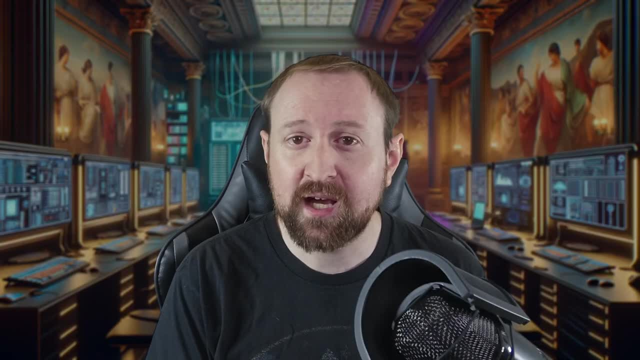 next time. That's all for me today. Hopefully, some or all of what I covered was useful and gives you ideas for how to get started in AppSec in 2024.. If you feel like I missed a great resource, please mention it in the comments below If you enjoyed the video and found it. 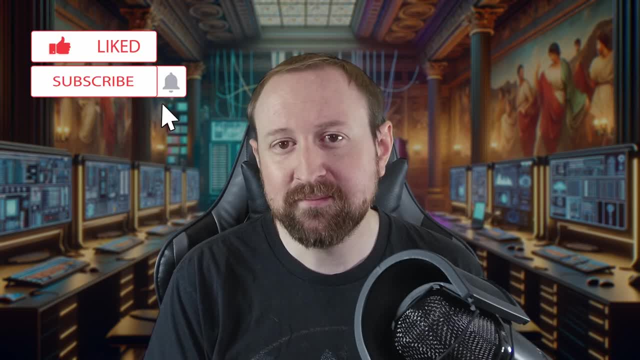 informative. please consider giving it a like. subscribe to the channel and I'll see you next time.